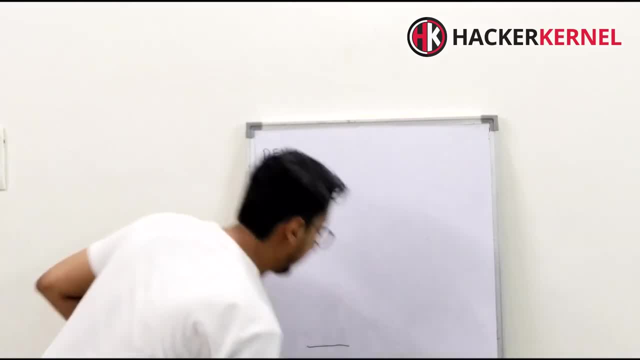 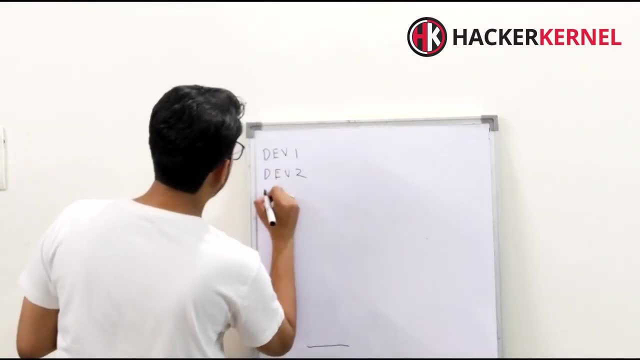 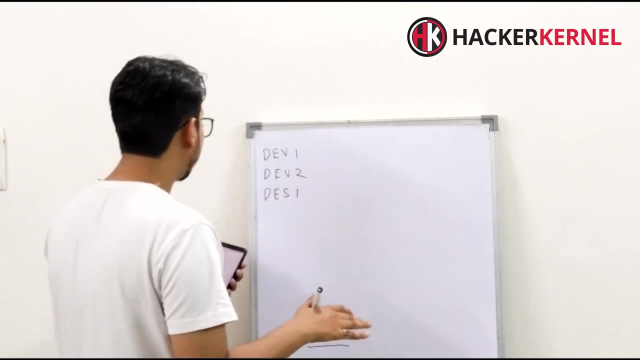 and then there would be dev- uh, let's, let me give more space over here. um, then there would be dev two. then there would be a designer one. for the sake of simplicity, we will only take three people, but in a real case scenario there would be more people, as there would be project manager involved. two testers wouldn't be involved. 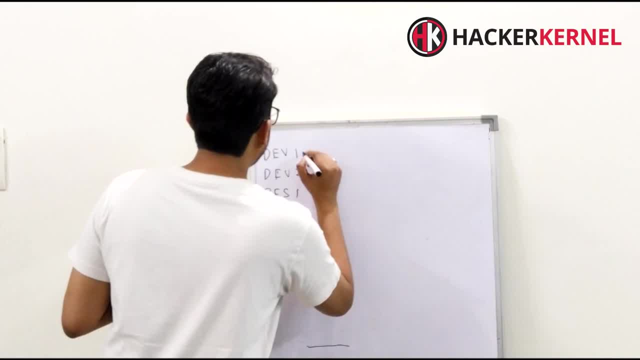 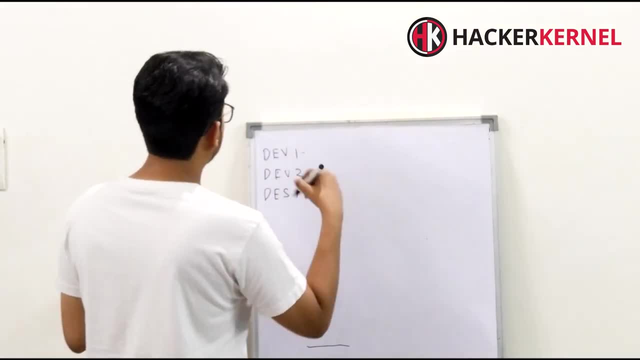 and all those kind of stuff. uh, so let's say, firstly, we need to calculate the, the salary you would be paying to these guys. so dev one is a average resource with a salary of twenty thousand rupees per month. dev two is a junior resource with a salary of 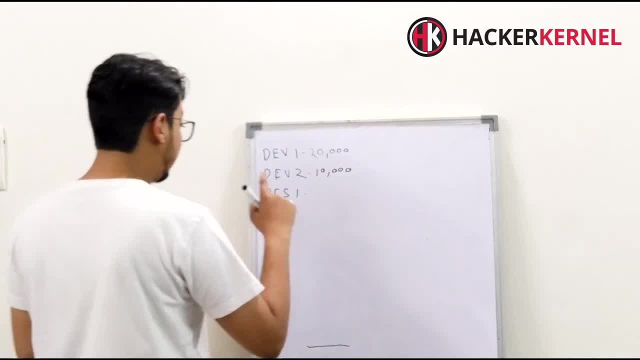 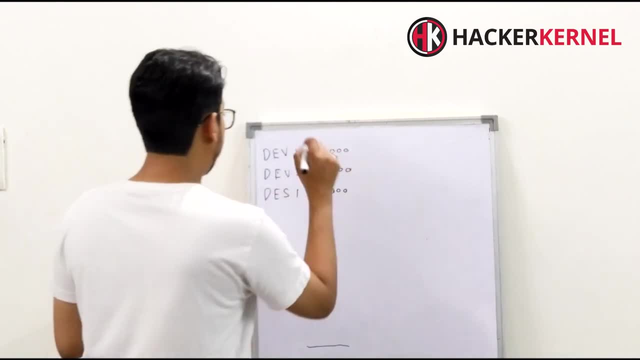 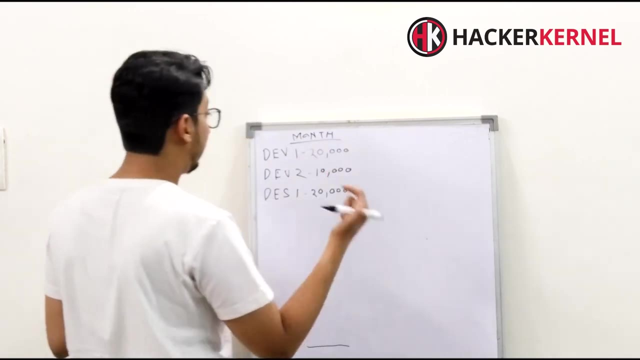 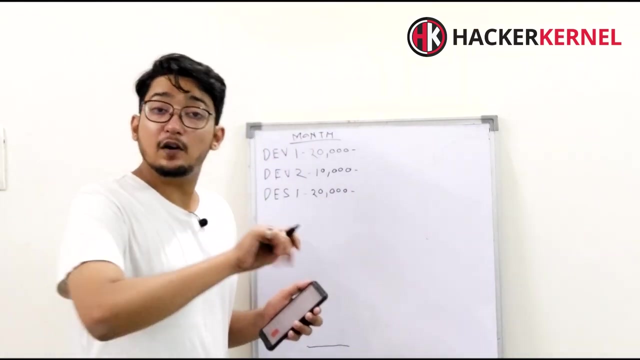 ten thousand rupees per month. design designer one is an average resource with a salary of twenty thousand rupees per month. so these would be the monthly salary. these would be the monthly salary of these people. right now. we need to estimate per day cost of these guys, as these guys will not be working monthly on this project. let's say: 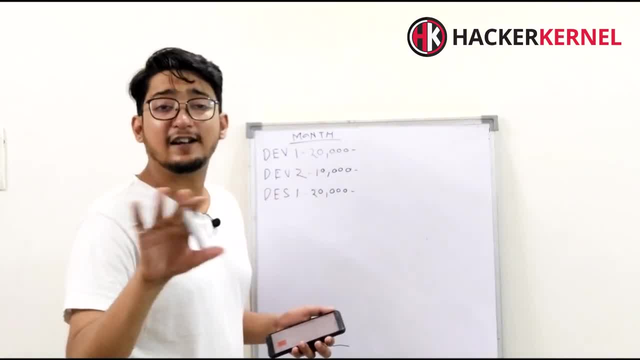 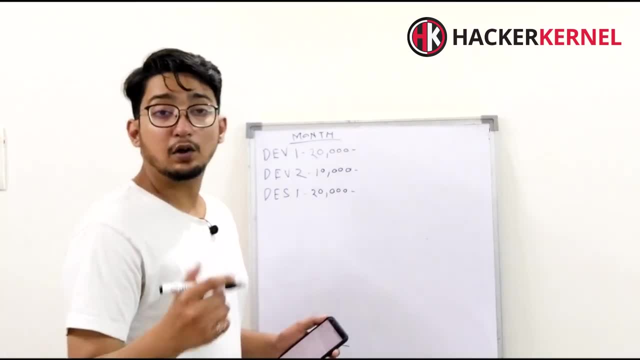 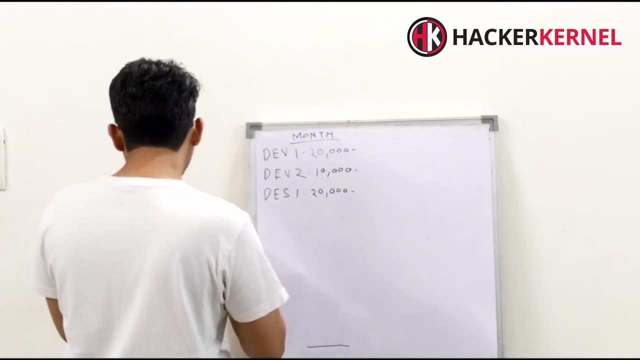 designer work. designer work only involved 10 days, so i do not, i do not want to calculate for the rest of 20 days, i will only calculate for 10 days. that's why it's very important to calculate per day cost. let's say, developer one per day cost would be 20 000 divided by 30. so if you divide by 30, that is also correct. but i do not tend to divide by 30 because in a month there would be certain working days and there would be certain holidays. so what i do personally do, is i divide by 26. i assume that there would be four more holidays, which would be sundays or 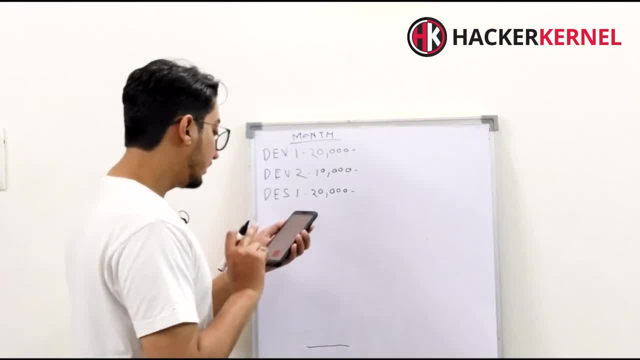 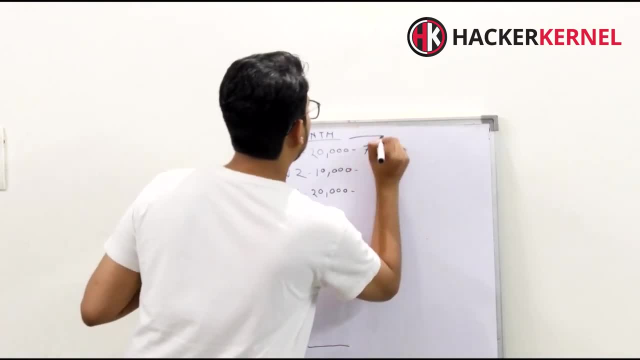 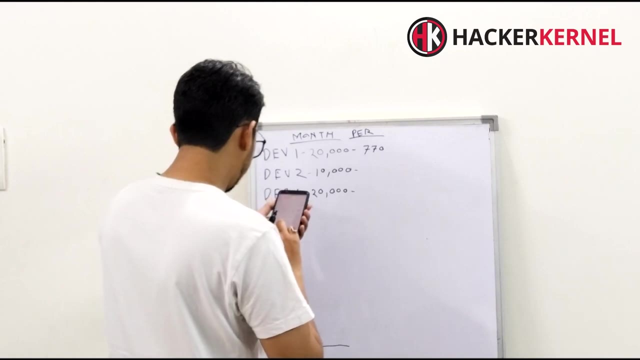 something else and i need to pay for those holidays, right? so then the per day cost would be estimated as 770 per day. so this would be the per day cost, correct. dev 2 would be for around 10 000 divided by 26. 10 000 divided by 26, it would be 390 rupees. 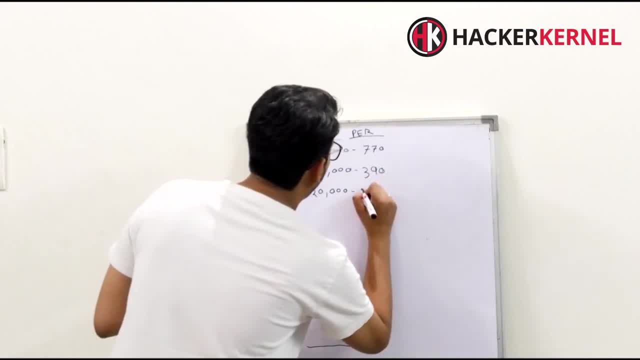 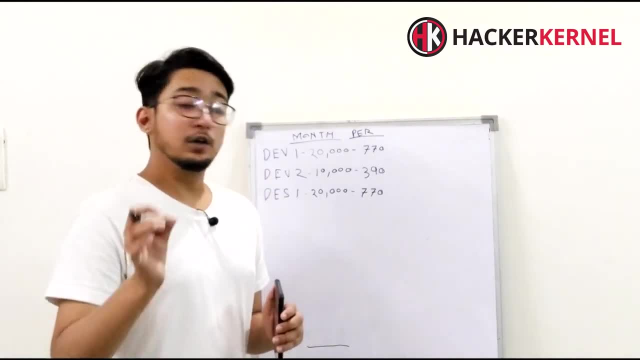 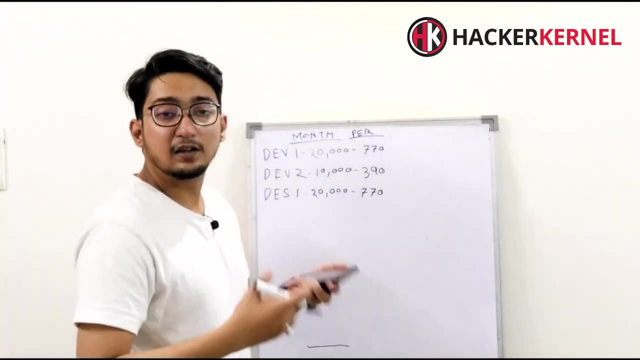 per day designer. one would be the same as 7, 70 rupees per day. this would be the per day cost you would be paying two these guys as a salary, right? uh, now, if a person, if any other person, would, what he would do is he would just add up these, add his margin and give that cost to the 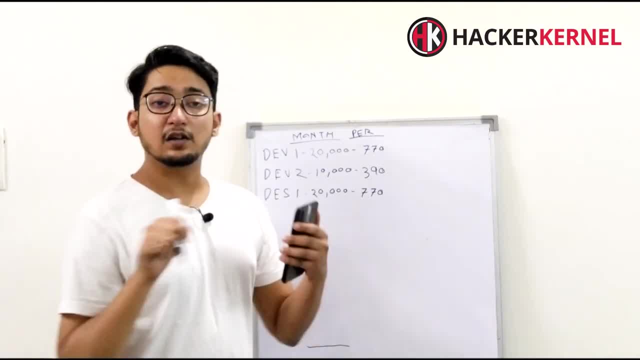 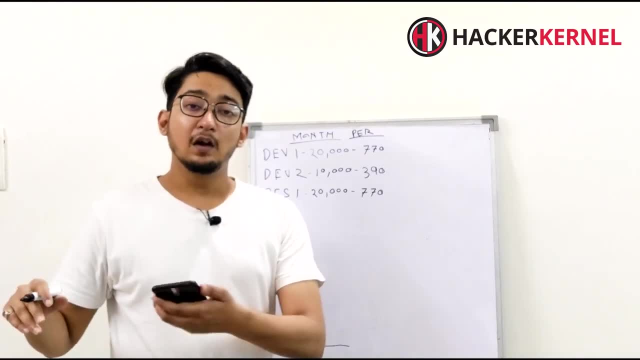 client, but that is not correct. as to set up this company, you have invested a lot of money- money you are investing every month in equipment. you have bought some computers, you have bought some. you have some real estate, you have some admin costs and all those details. so you need to add up. 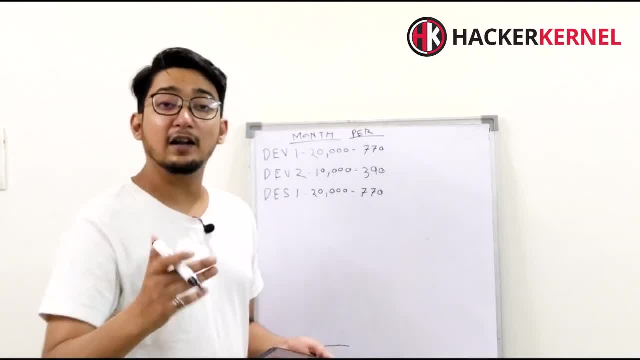 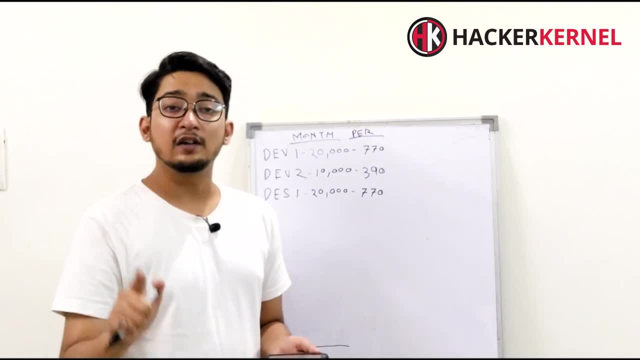 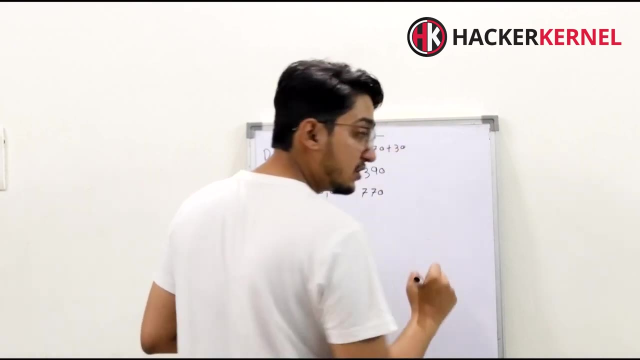 those costs as well as those costs would be end up eating your profitability, which is very bad. as i always say, profit is the oxygen in which every organization survives. so, firstly, what i usually do is i plus 30 percent as a markup cost. as a markup cost, this markup cost would be for: 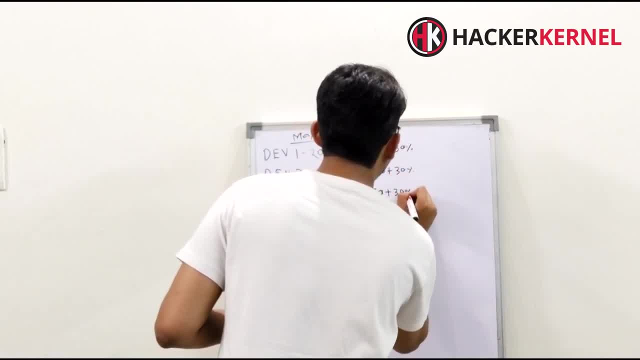 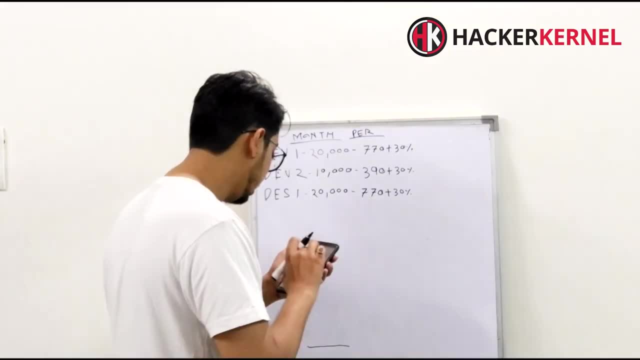 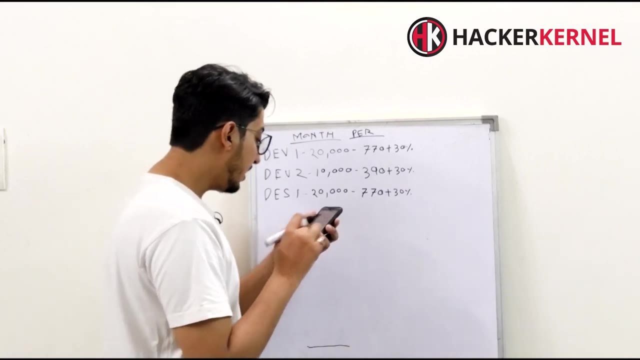 the admin, things like hosting these people, cost of the computers, cost of depreciation costs and all those details, ideal state infrastructure costs and all those details. so let's say 770 plus 30 percent, it would be like 1000. so it would be the markup cost would be. 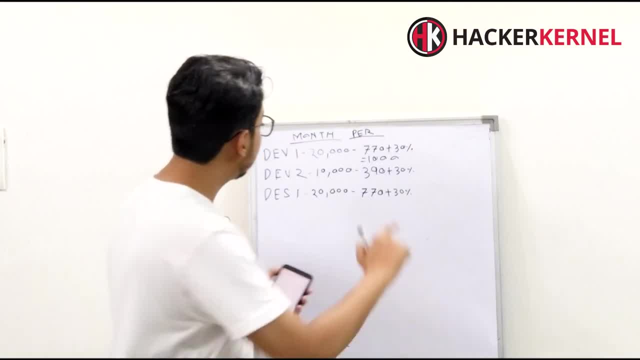 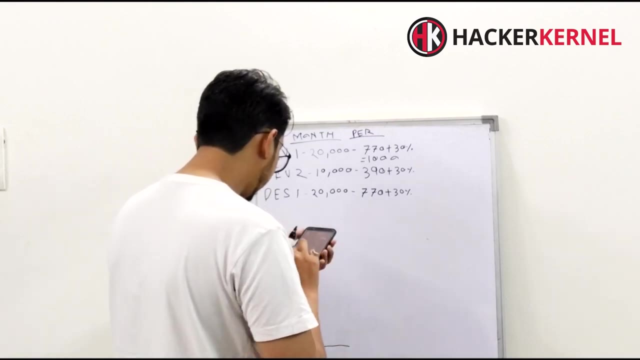 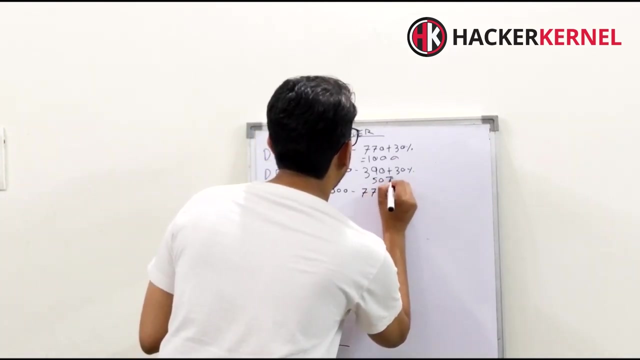 1000. so his per day cost, the original per day cost, is 1000 rupees. this would be the cost, which is which you are paying to this employee every day. now for this guy, which is the dev2, the junior resource, you would be paying like around 507. for the sake of simplicity, let's take 507, right. 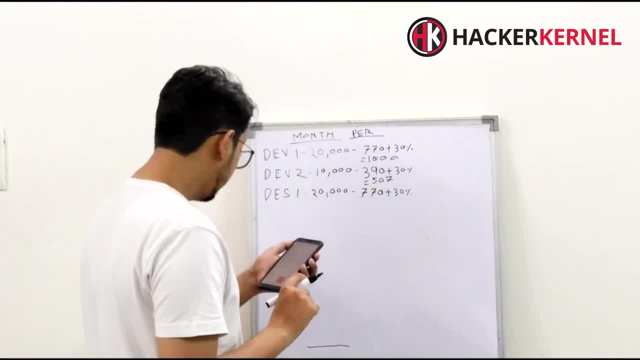 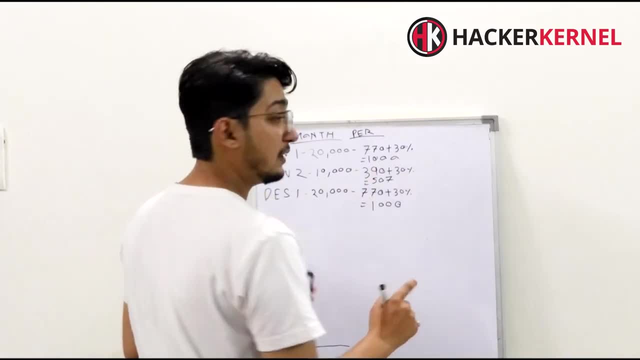 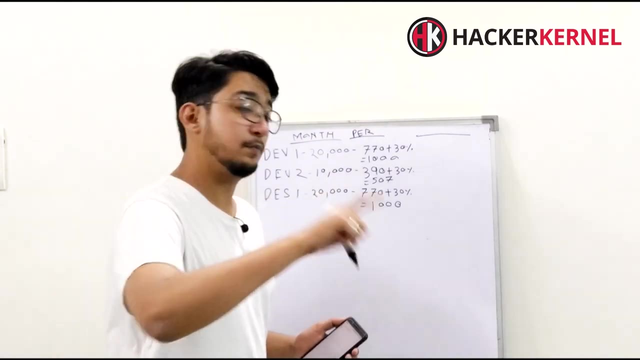 so this would be his per day cost. now for the designer one it would be the same as the dev1, which is 1000 rupees per day. now we would estimate how many days these guys are gonna work in this project. let's say these guys are gonna work in this project for. 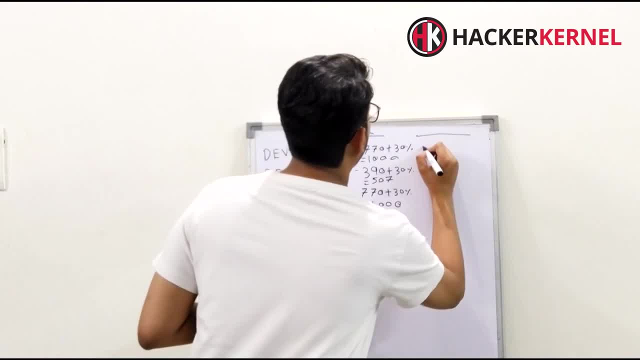 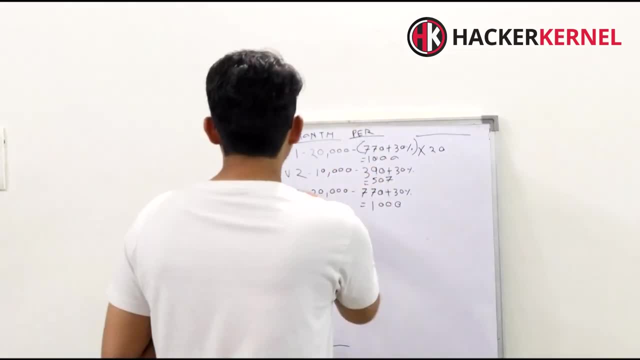 my dev1 would be working for around 30 days. so, whatever the sum of this is, you would be paying for the dev1, which is 1000 rupees per day. so this would be his per day cost. i would be multiplying it with 20.. my dev2 would be doing some admin work, admin area work and 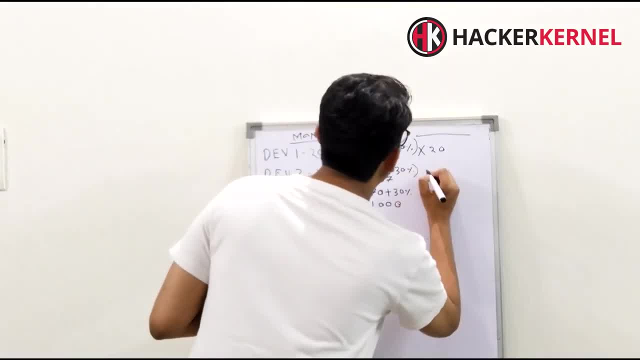 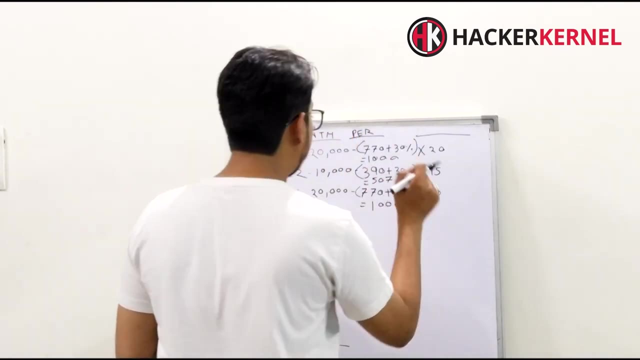 some. he would be helping my dev1, so he would be working for around 15 days. for the sake of simplicity, and designer work would be working for around 10 days, right, so i would simply. what i would do is i would just simply multiply 20 into 1000, which would be: 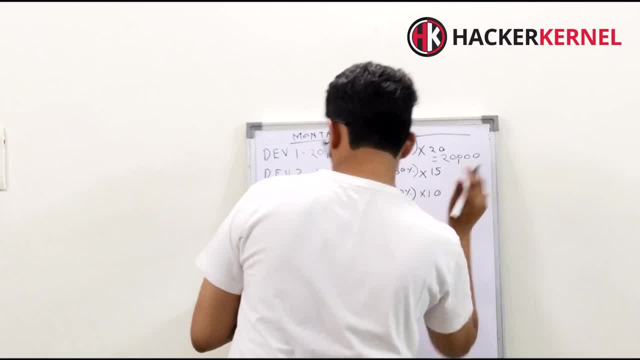 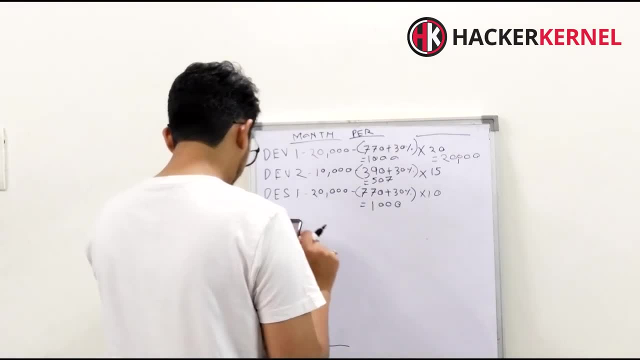 20 000 if i am correct. i am very bad at maths but i can use excel very perfectly, so i was correct. it is 20 000 rupees. so 20 000 would be the cost of my dev1. now the cost of my dev2 would be 507, 507 into come on 407 into 15, which would be 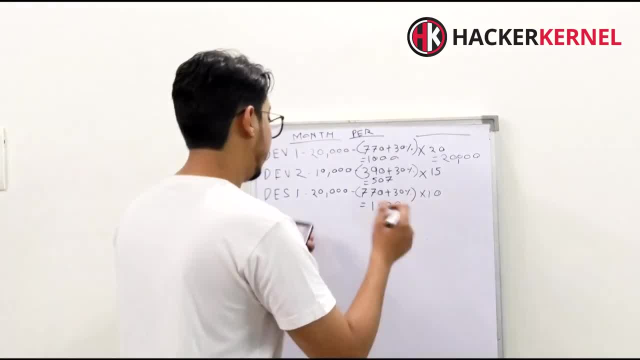 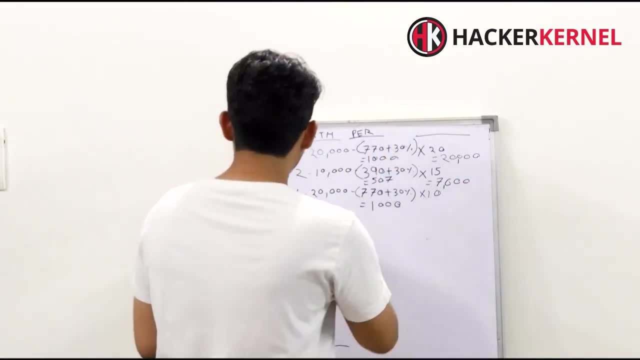 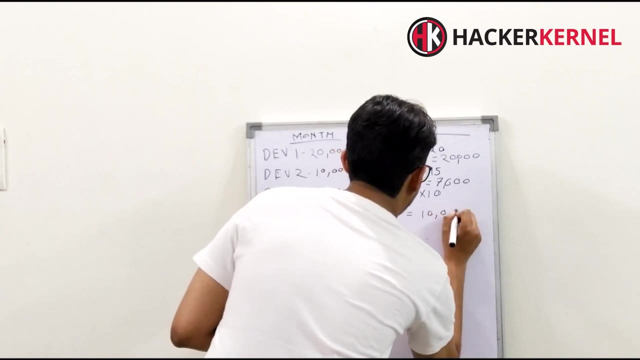 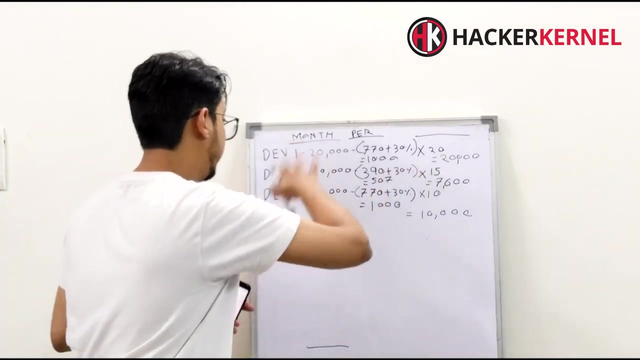 uh, 7605. for the sake of simplicity let's round it off to 7600 rupees, correct? same would apply to my designer one. his would be around 10 000 if i am correct, and i am correct for this. so these would be the per day cost for my per project cost for these, for three resources. now let's calculate. 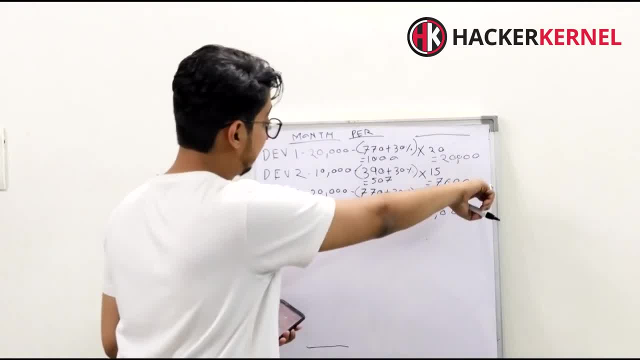 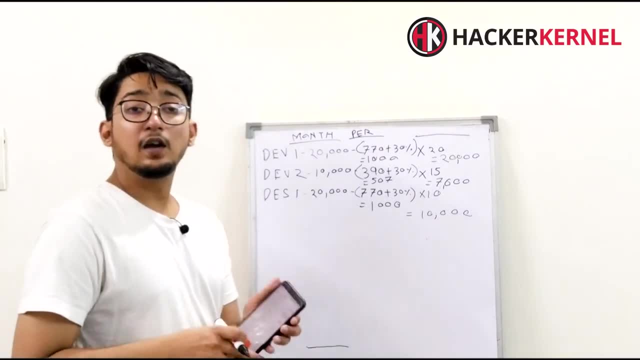 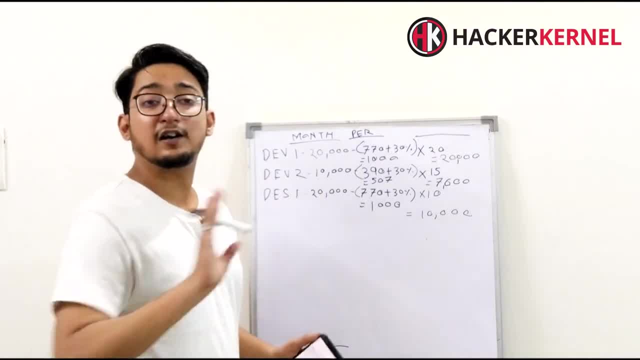 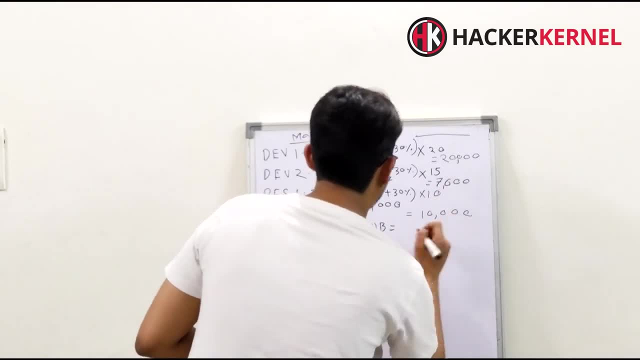 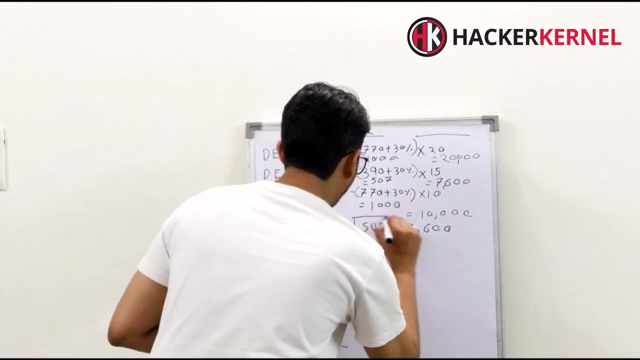 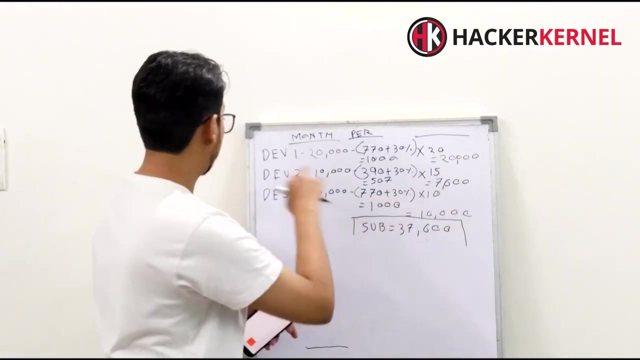 in order to get this project done. in hindi we say so. it would be around the sub total. sub total would be thirty seven thousand six hundred rupees. this would be my sub total. this would be- i am adding up this with this- with this, so that dev1 would be involved. for 20 days, dev2 would be involved for 50 days, design one. one would be involved for 10 days. so my sub total cost would be 37 600. now the most important part is to add up my profits. every organization estimates its profit differently. some do it with 20 percent, some 30 percent, some 40. 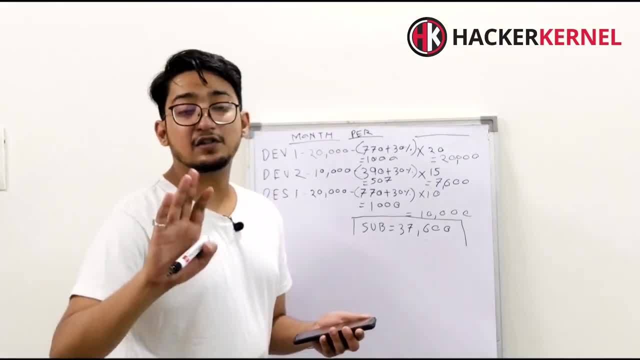 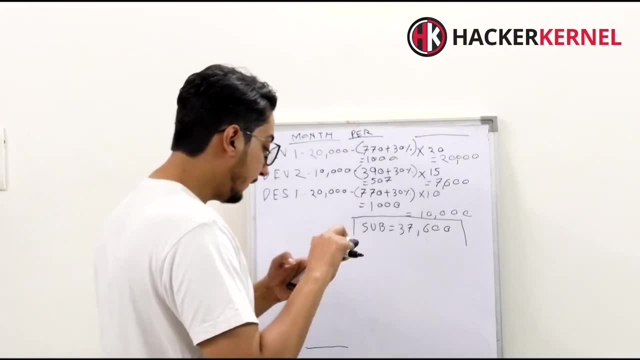 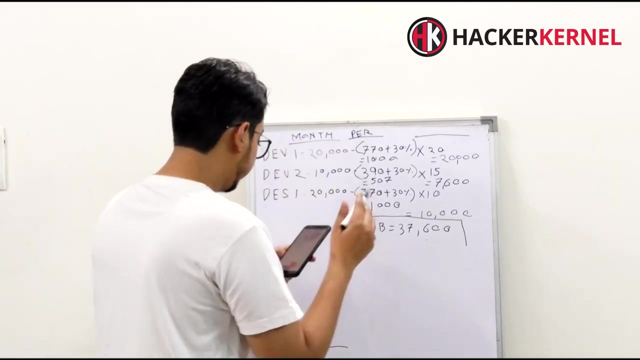 let's say, for the sake of simplicity, we are a new organization and we only charge 30 as our profit. so 37 600, uh plus- give me a minute- 37 600 plus 30 is my profit. it would be, um, it would be, total of. 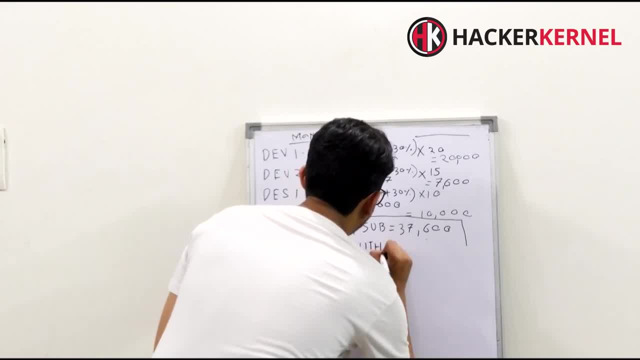 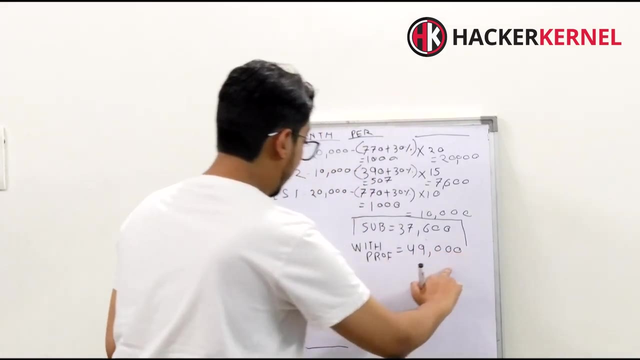 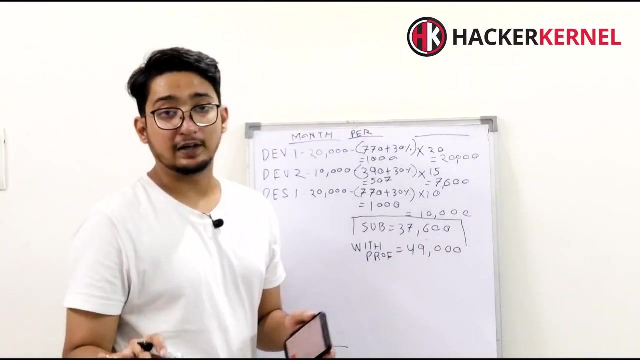 with profit. so with profit, prof. for the sake of simplicity, again 48 880. let's round it off to 49 thousands. so 49 000 would be the cost with profit. this is the cost which i can give to the client, but but as we live in india and most of the clients would, 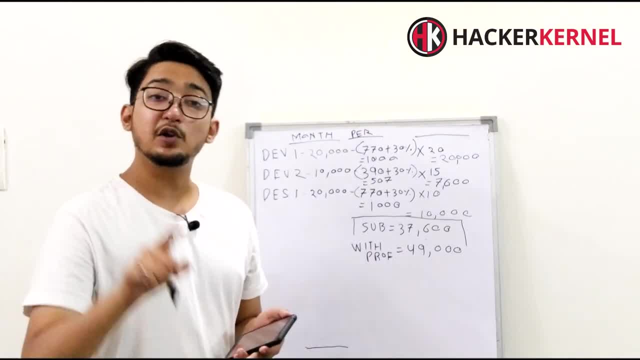 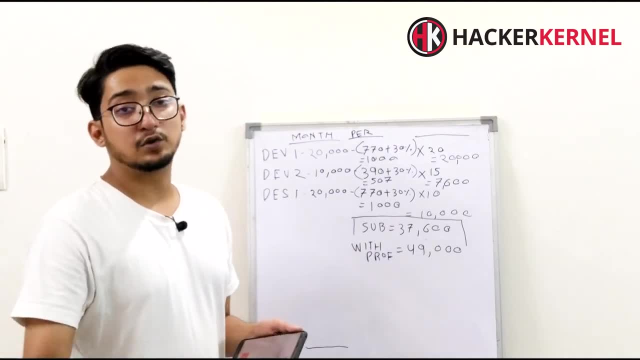 uh, negotiate with you. so you need to be really smart. you need to add a negotiation add-on which would give you a extra question in which you could, uh dis give discounts to the client. let's say, if client asks you for some discount, you can give a five percent discount or ten percent discount. 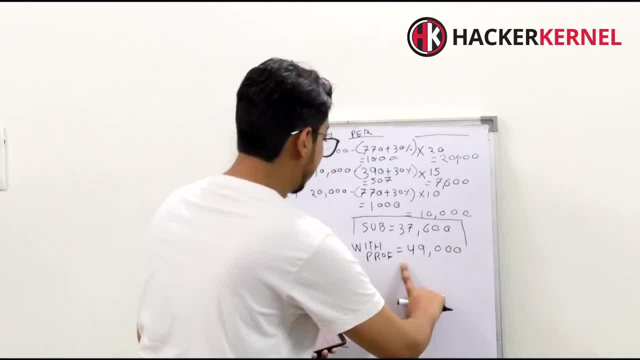 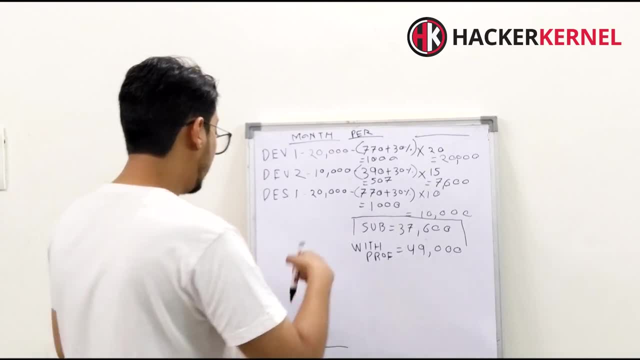 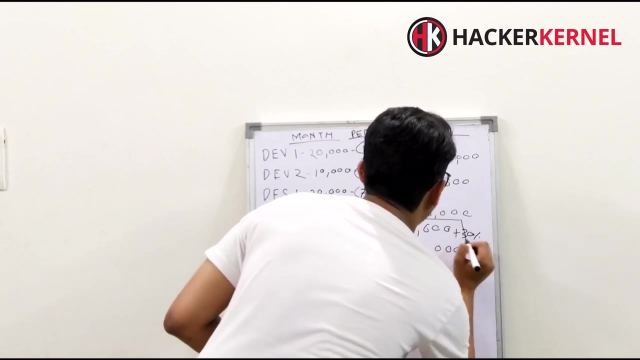 if you started to give discount from this price then, uh you, your profit margin would suffer. so i do not recommend to give discount from this price. what you could do is you could have a negotiation add-on which would be: uh, let's say, i would just add 30 percent as profit over here. 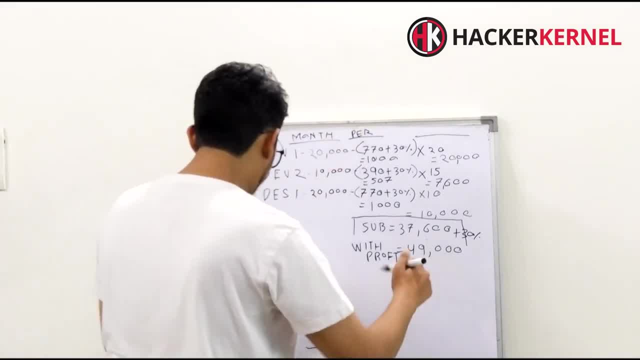 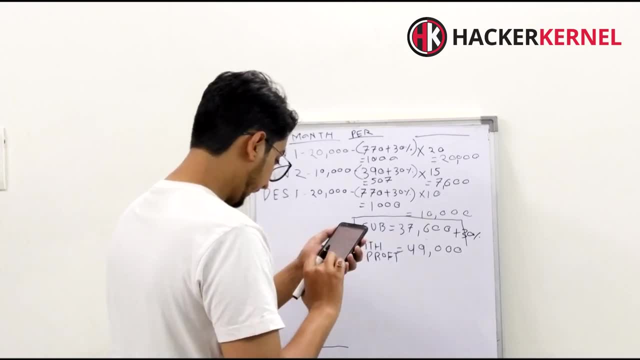 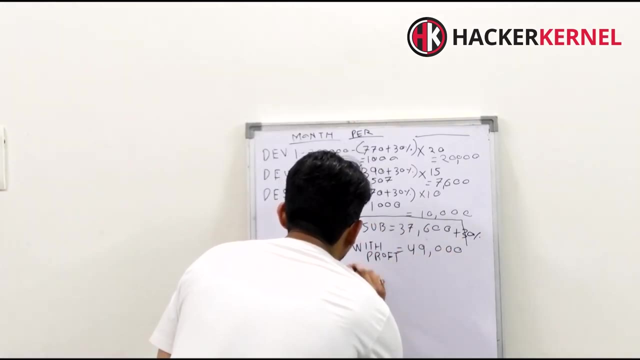 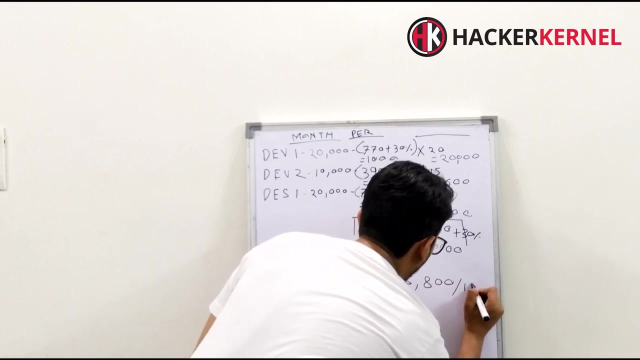 and then, with profits, profit, you could add another 20 percent as your negotiation add-on. so four, nine, double zero plus twenty percent would be five, eight, eight hundred, so with, so this would be your final price, final cost, which would be fifty eight thousand eight hundred. i and r. so this would be your final cost and this 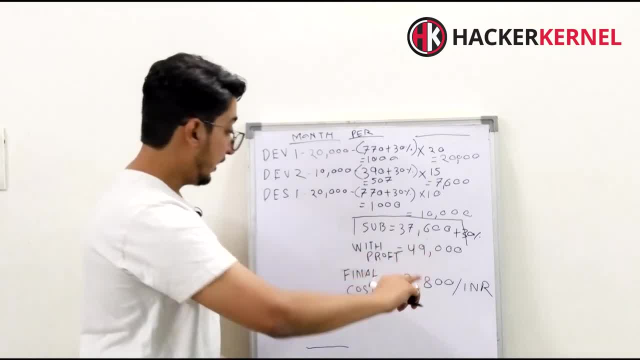 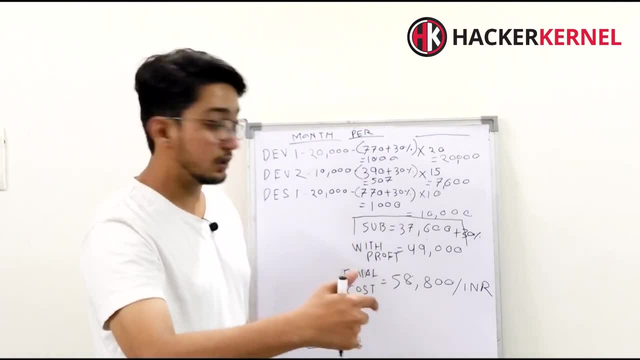 is the cost of the project you should give to the client. and then, once you give this cost, you would be having certain- uh, what we call a cushion negotiation question, which would be of ten thousand rupees or twenty percent. if client asks for a discount, you could give that discount to.